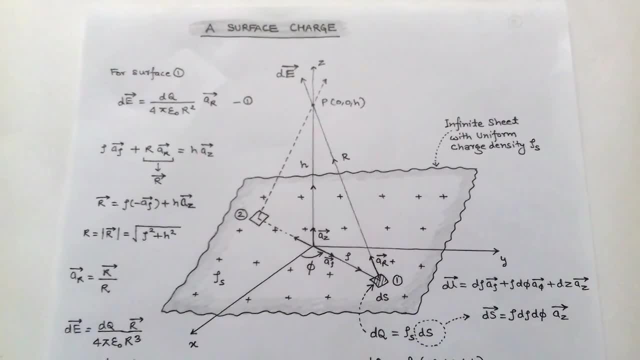 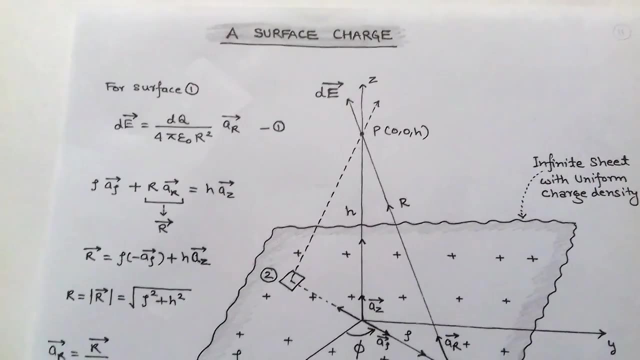 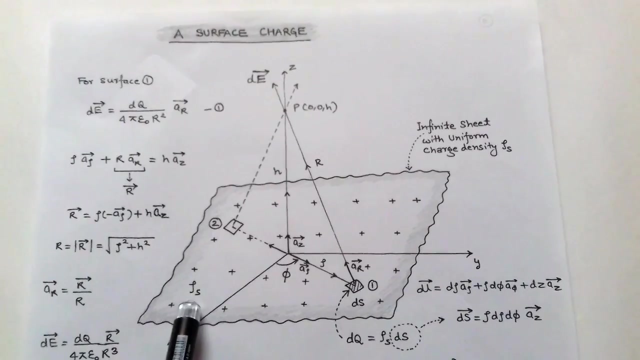 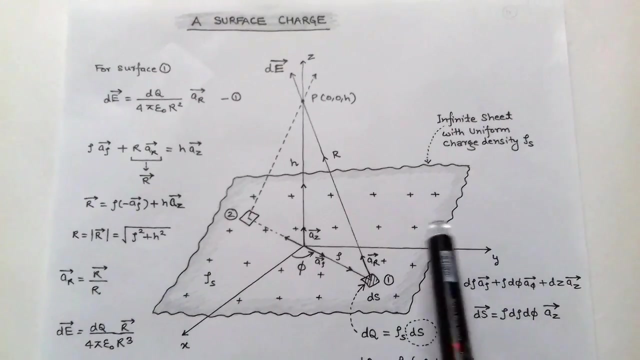 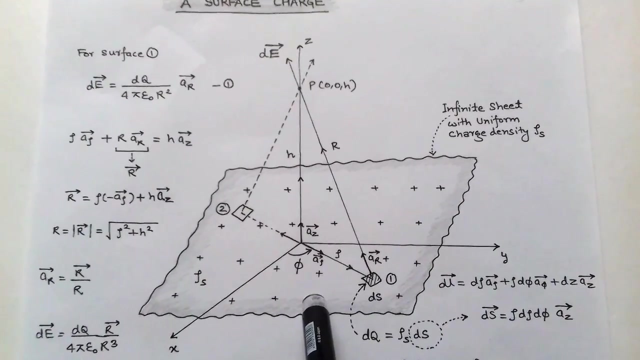 Surface charge. Here we consider XYZ plane and on this XYZ plane we consider an infinite sheet with uniform charge density: Rho S. So here this is a infinite sheet having a uniform charge distribution. Here the positive charge is uniformly distributed, which having a surface charge density Rho S. 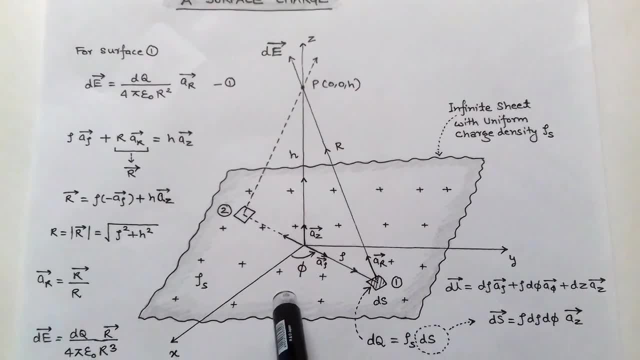 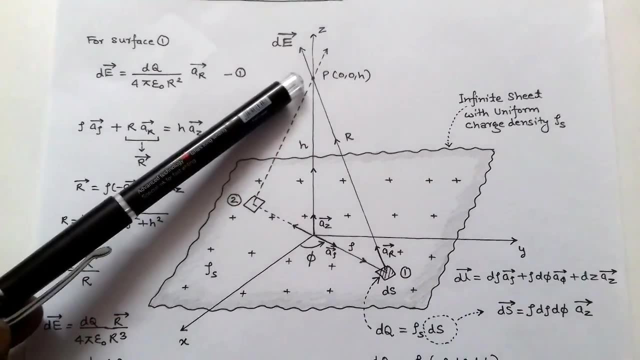 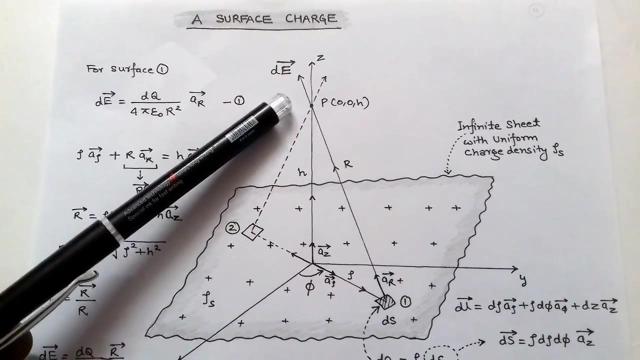 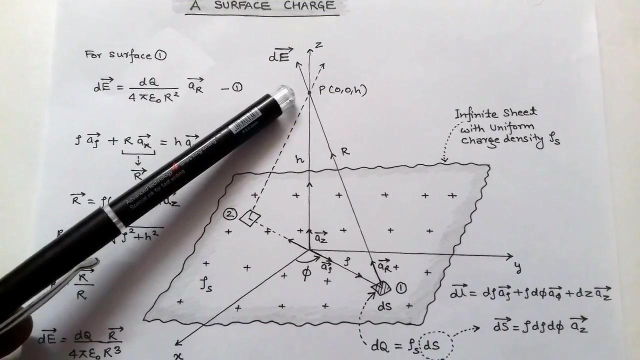 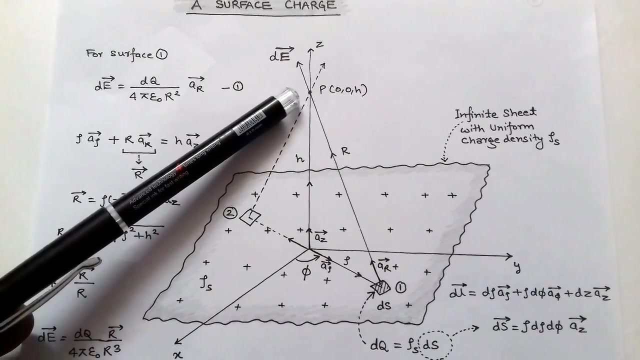 Now, due to this surface charge density, Rho, S, or due to infinite sheet, we have to determine the electric field intensity at point P. This point is situated on Z axis, So the coordinate of this point is: means this point is on Z axis, means X and Y coordinate is 0 and this point having some height. 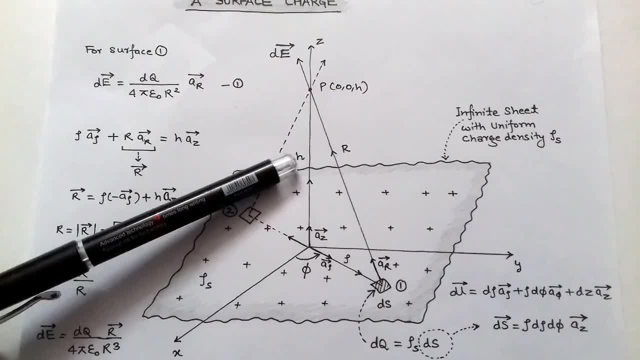 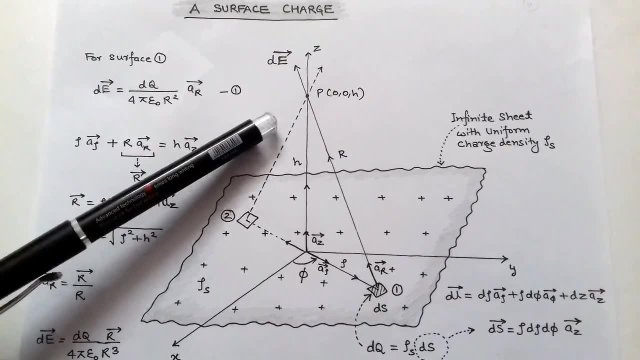 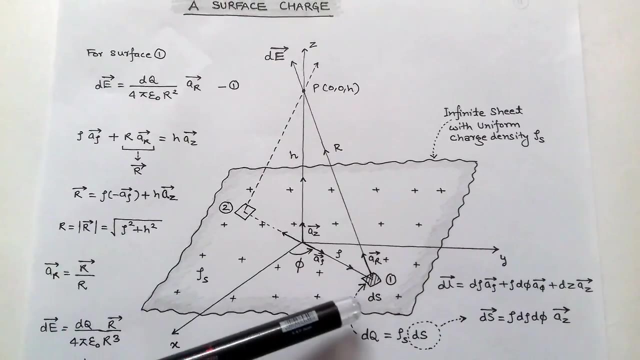 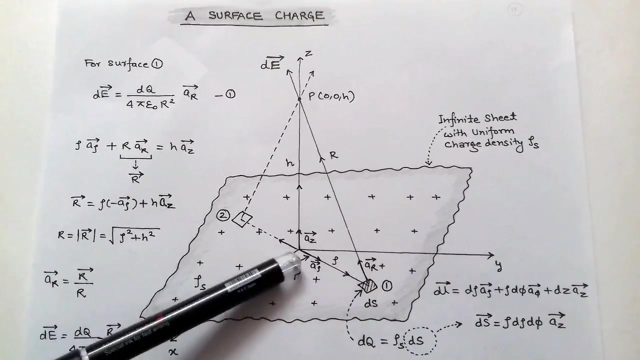 So this height is H, So the coordinate is Now. the first step is on this infinite sheet. we consider small differential surface, ds, and mark with 1.. This ds is at some distance, Rho, with respect to origin, And this Rho distance having a unit vector. 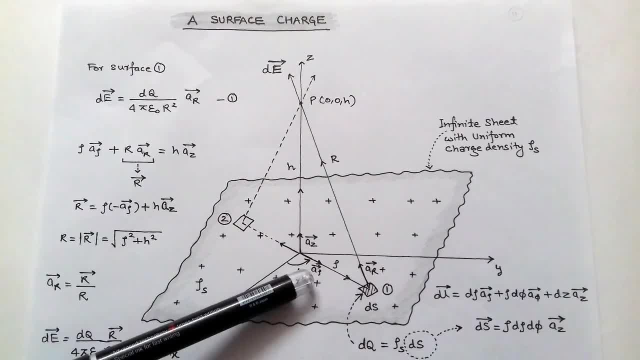 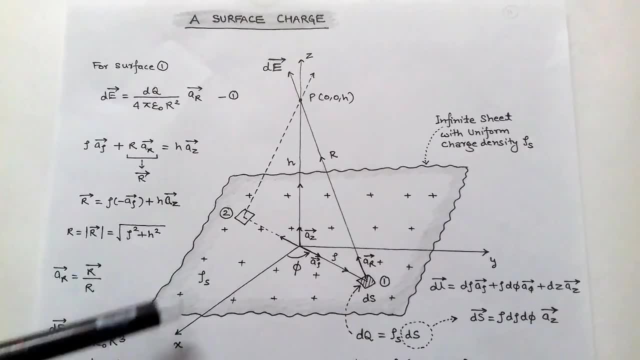 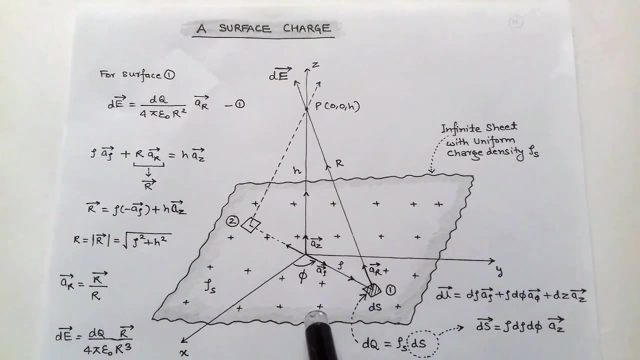 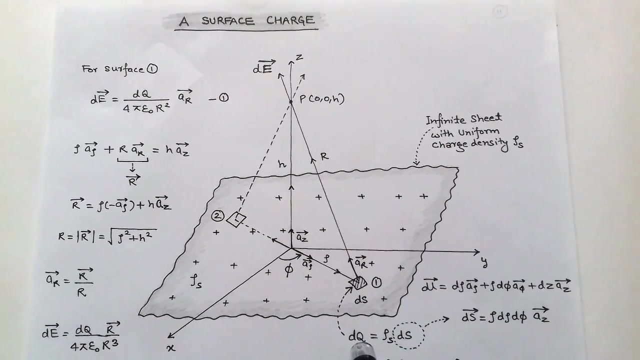 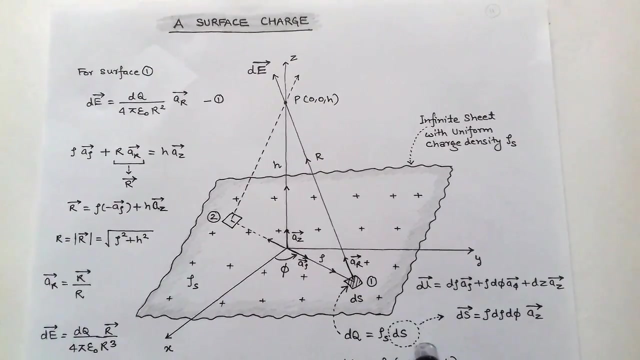 E, Rho. This Rho makes some angle Phi with respect to X axis. So here we consider a circular cylindrical coordinate system. Now this differential surface ds having a small charge, dq. So dq equals to Rho, S into ds. Now what about ds? 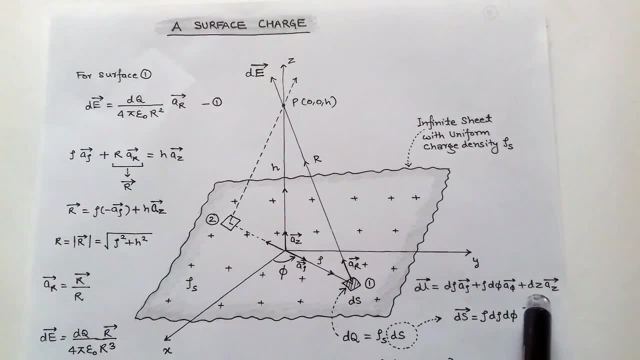 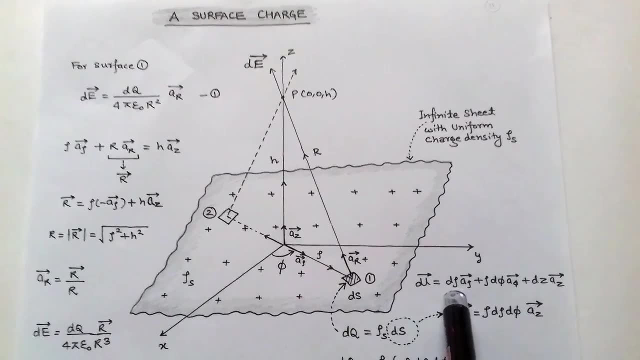 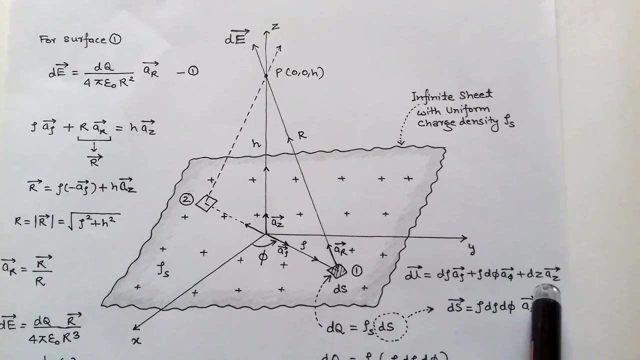 So ds value can be calculated using differential length in cylindrical coordinate system. So dl in cylindrical coordinate system is: d Rho unit vector Rho plus Rho. d Phi unit vector Phi plus dz unit vector z. Since this infinite sheet is situated at z equals to 0. 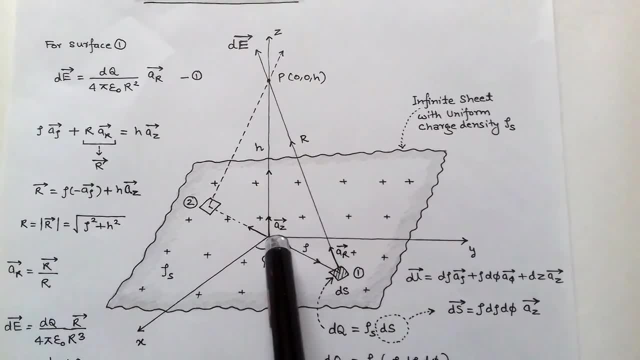 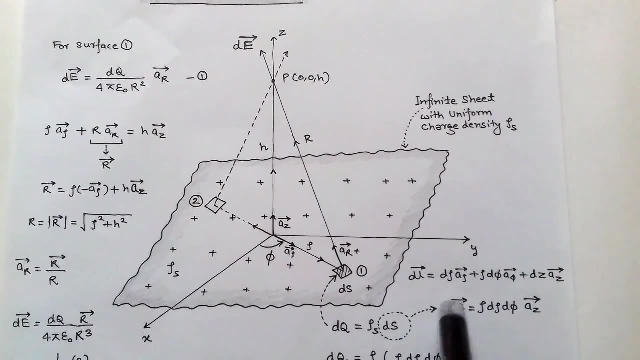 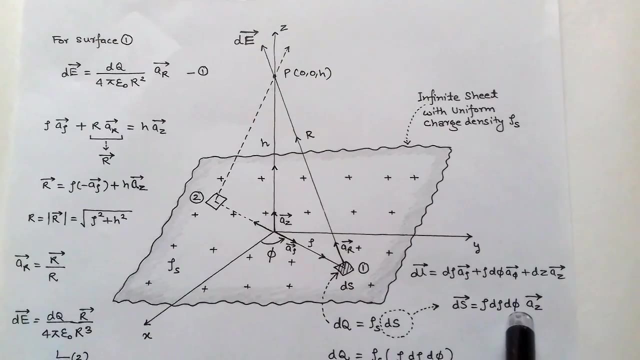 that is, xy plane. So this infinite sheet having a normal direction, that is, towards z direction. So differential surface in the direction of z is equals to d Rho into Rho d Phi in the direction of z. So the magnitude part of ds value. 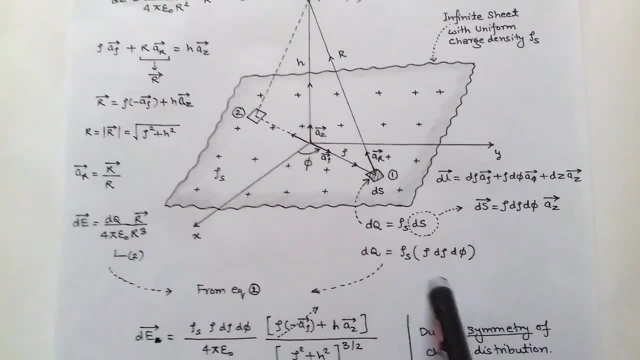 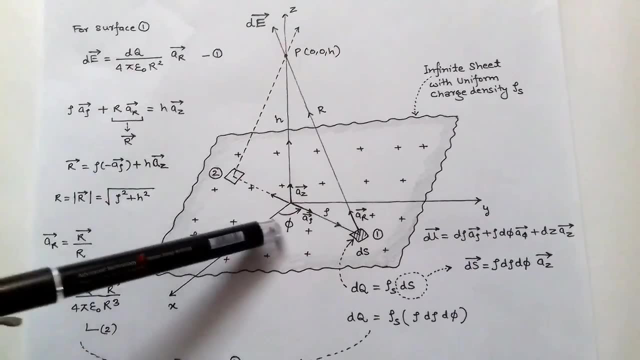 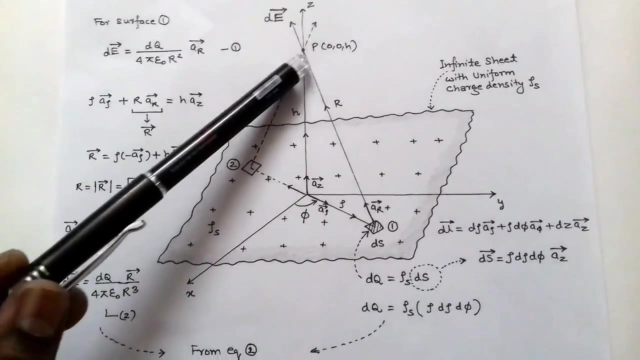 is Rho d Rho into d Phi. So in place of ds we can write Rho d Rho into d Phi. Now now from here, since ds having a distance of Rho. Now this point, P is at some distance with respect to ds, that is. 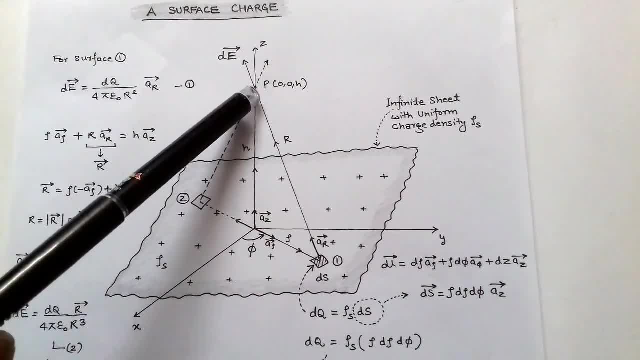 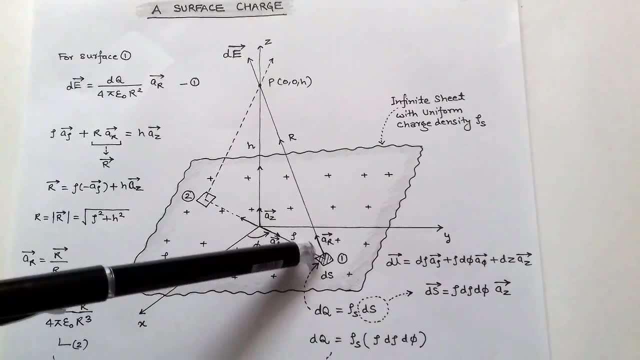 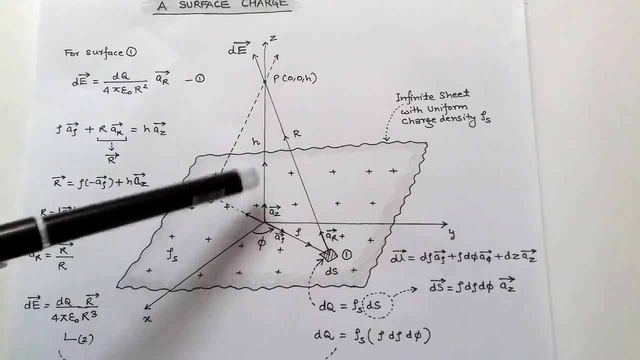 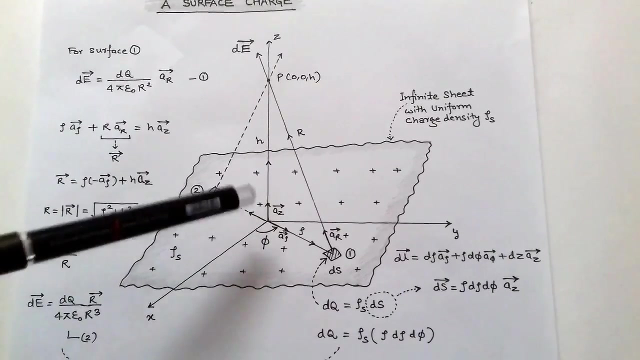 R and this point having some height, h. Now we take all the unit vectors: unit vector Rho and unit vector R, capital R, that is between ds and point P, and unit vector z towards z axis, that is between point P and origin. So here we. 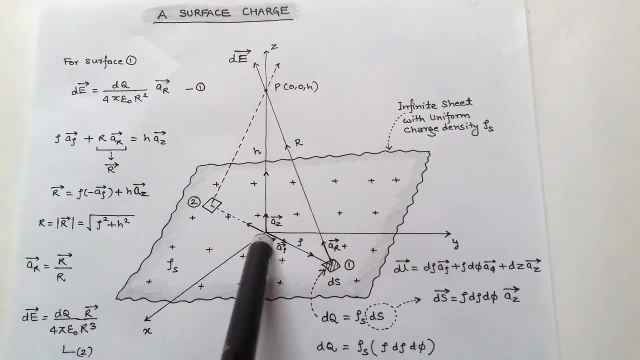 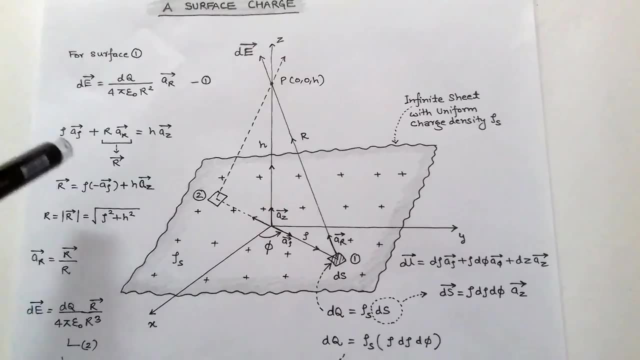 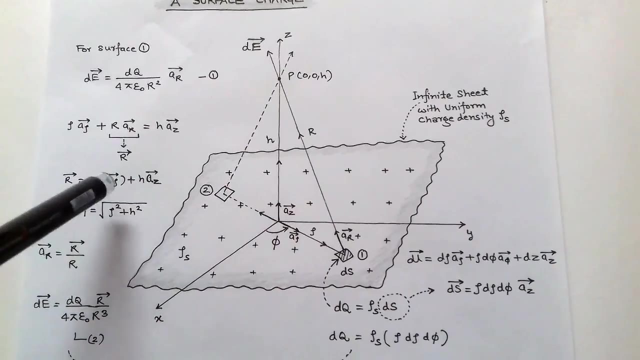 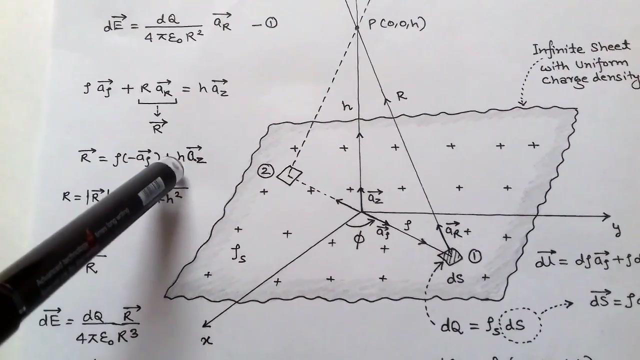 using a vector sum method. so Rho unit vector Rho plus R unit vector R equals to h unit vector z. and here, in place of R unit vector R, we can write vector capital R, so capital R equals to Rho minus unit vector Rho plus h unit vector z. 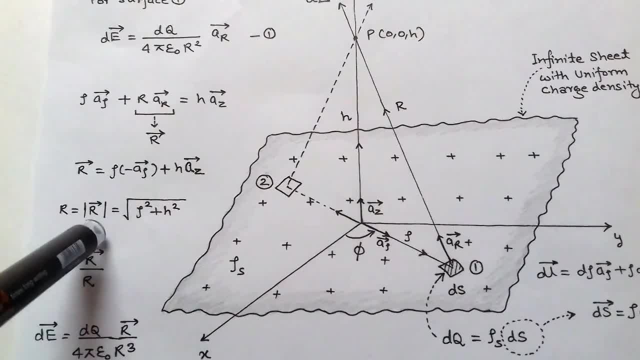 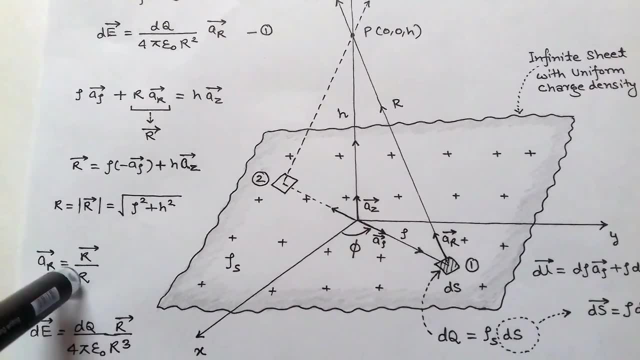 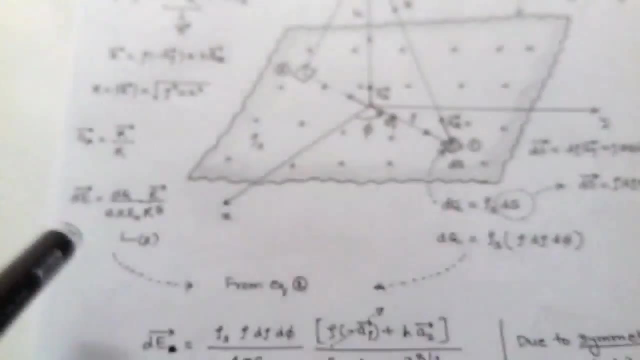 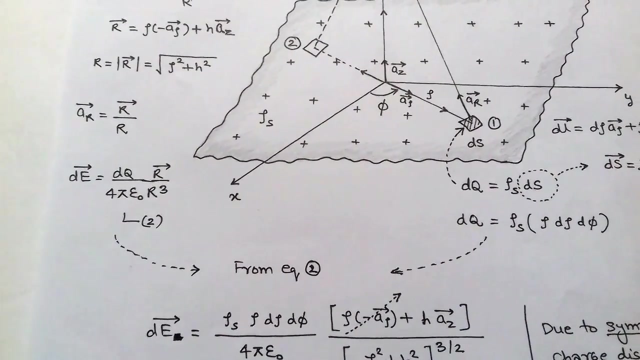 the magnitude of this, that is, R, is equals to under root Rho square plus h square. this unit vector, R, is equals to vector upon its magnitude. After putting this value of unit vector equation 1, we get dE, small electric field. dE equals to dQ upon 4 pi epsilon. 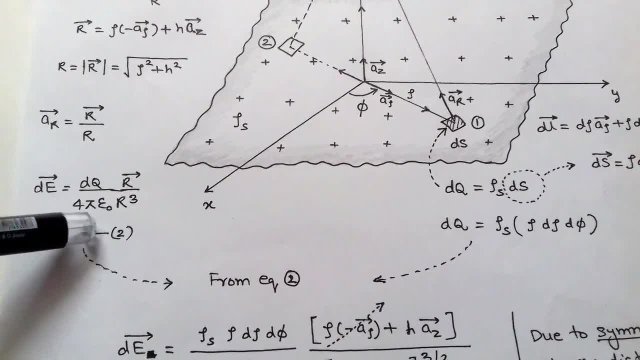 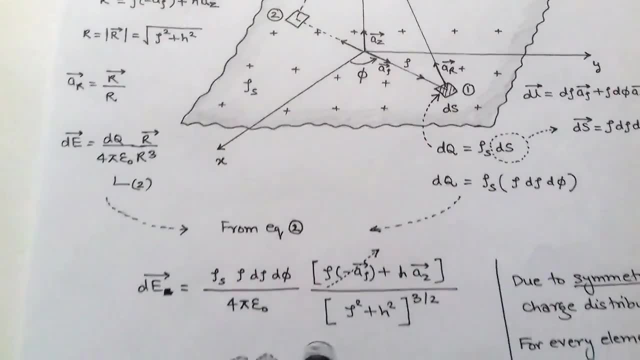 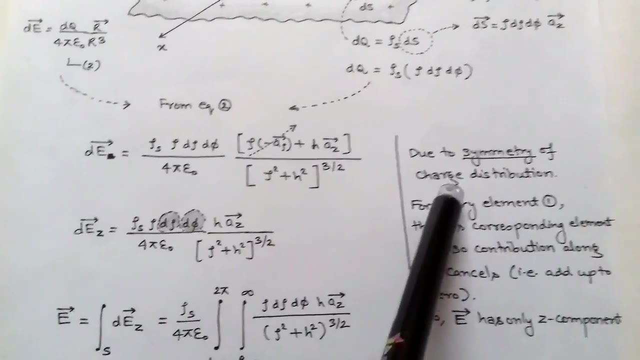 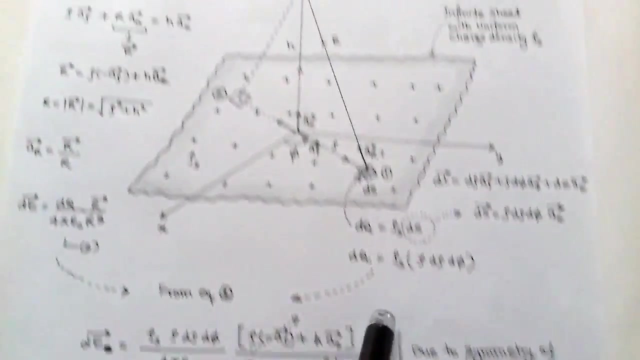 R vector R upon magnitude cube. So in place of dQ we can write Rho s into Rho, dRho into d phi. So after putting this from the symmetry point of view, for for a symmetrical chart distribution for every element: 1. 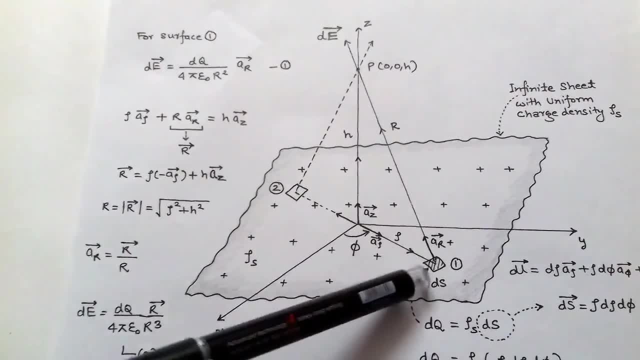 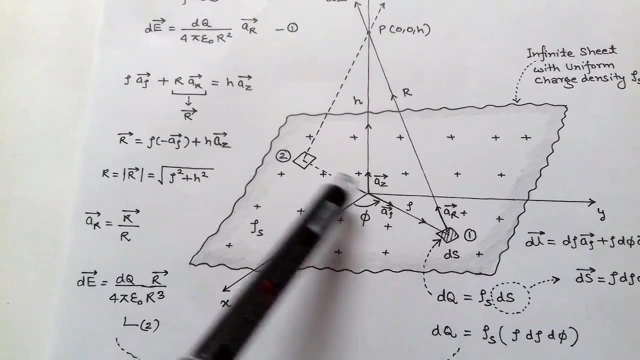 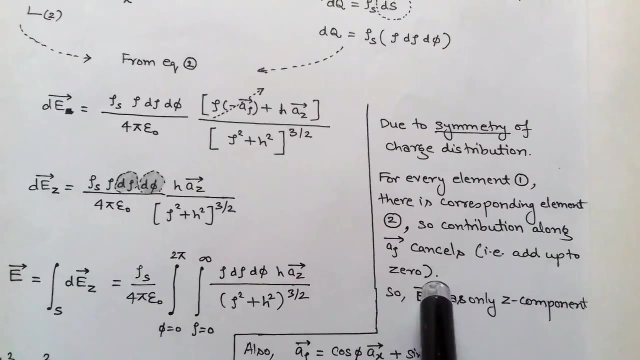 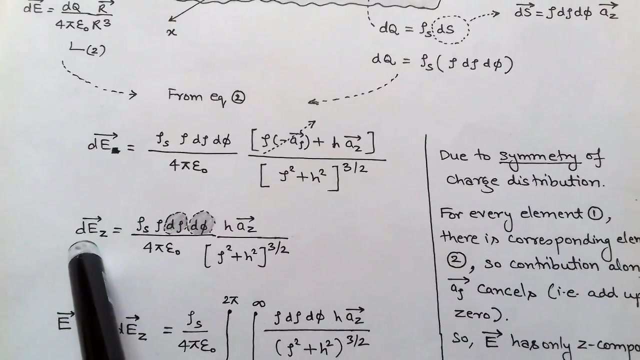 there is corresponding element 2, so contribution along A Rho, cancel, cancel, that is add up to 0. so electric field intensity has only z component. so due to symmetry, Rho component is 0, so so the electric field intensity has only z component. so here: 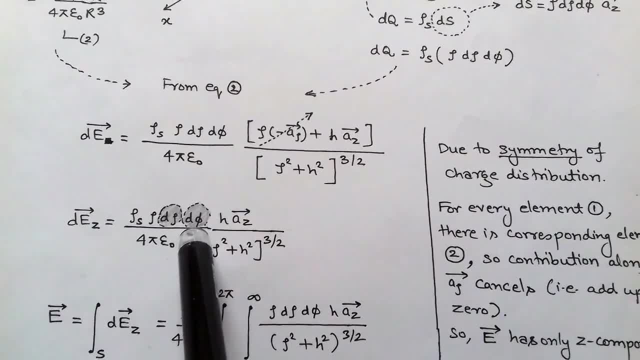 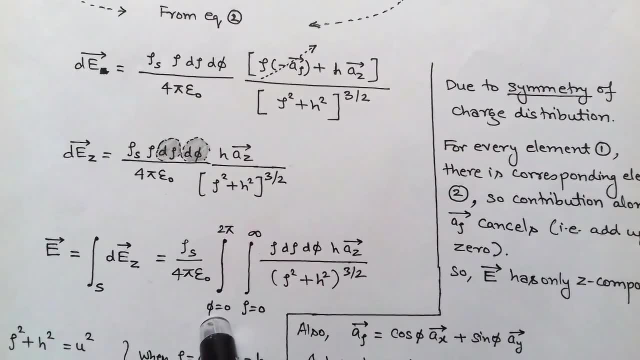 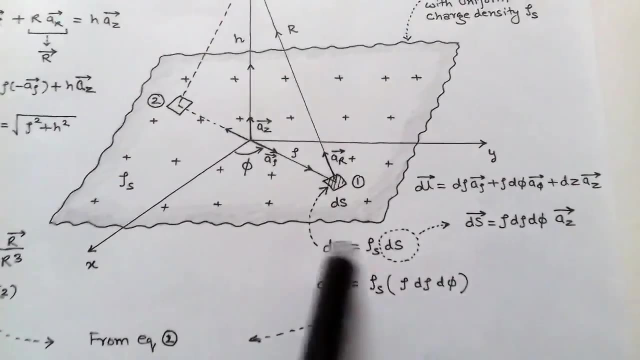 there is differential dRho and d phi. so we integrate with respect to Rho and with respect to phi. so there is two integration, one for Rho and second for phi. now the Rho, the limit of Rho. since it is infinite sheet, the limit of Rho is 0 to. 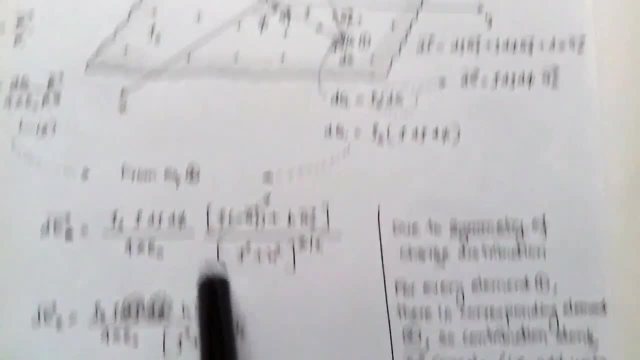 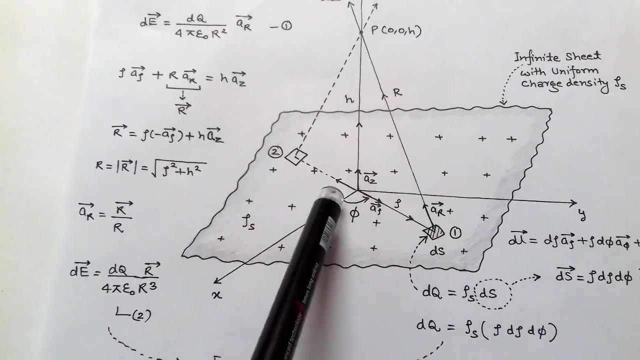 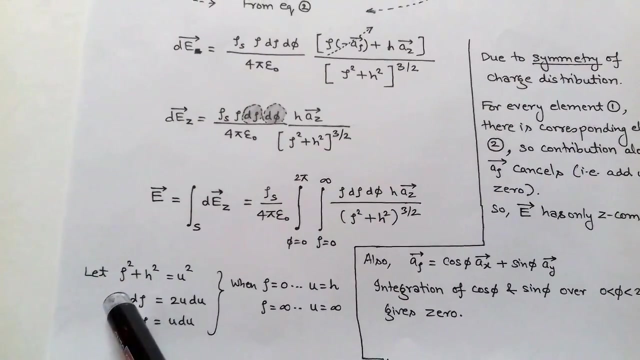 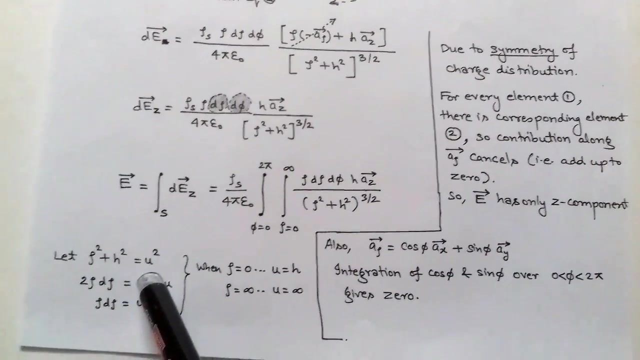 infinity, while the limit for phi phi is from with respect to x axis, that is from 0 to 2 pi. now we assume some value, that is, let Rho square plus s square equals to u square. we consider here this value should is equals to u square for the calculation of. 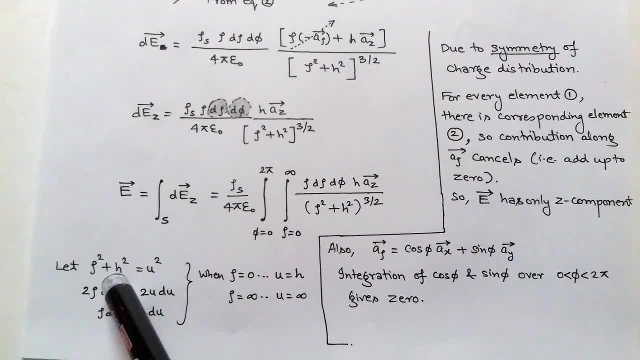 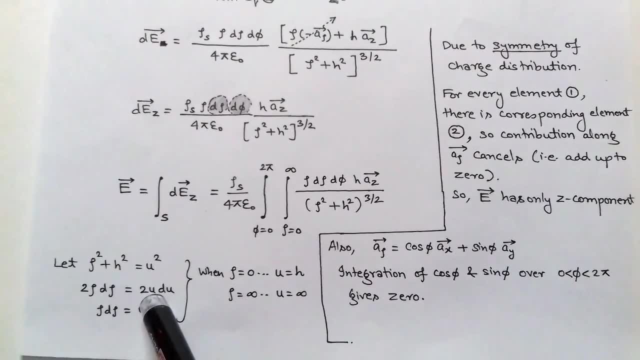 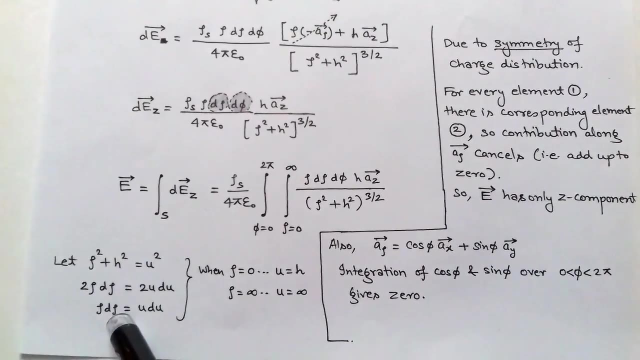 this integration. so h is constant. so the derivative differentiation, that is, 2 Rho d Rho equals to 2 u du and Rho d Rho equals to u du. so in place of d Rho, Rho d Rho, we can write u du. 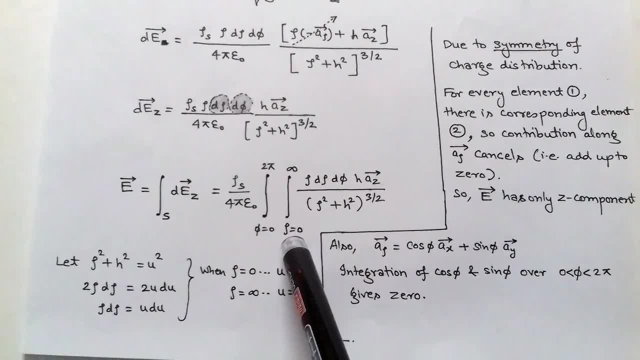 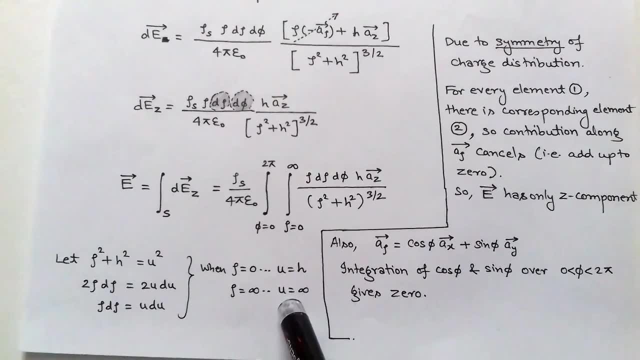 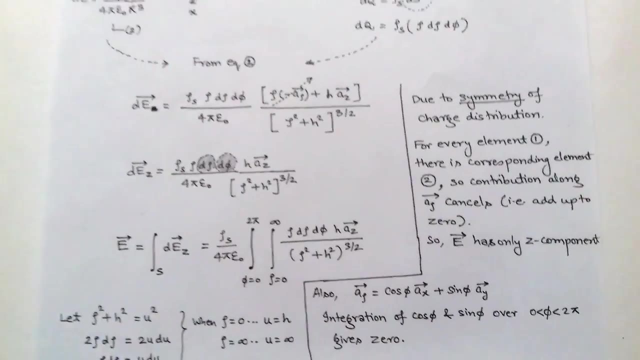 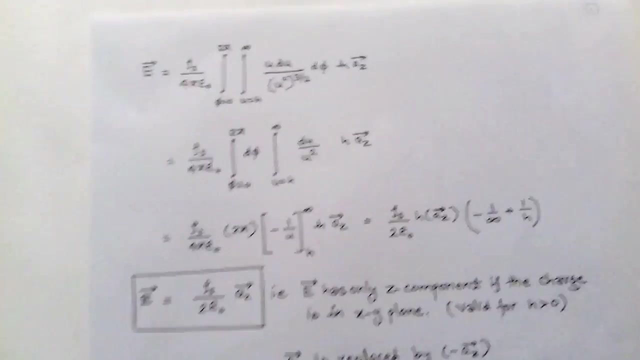 similarly, the limits can also be changed. so when Rho equals to 0, then u becomes h. when Rho equals to infinity, u becomes infinity, so the limits is changed. after putting this, we get a total electric field, e. now we have to calculate this, we have to integrate it. 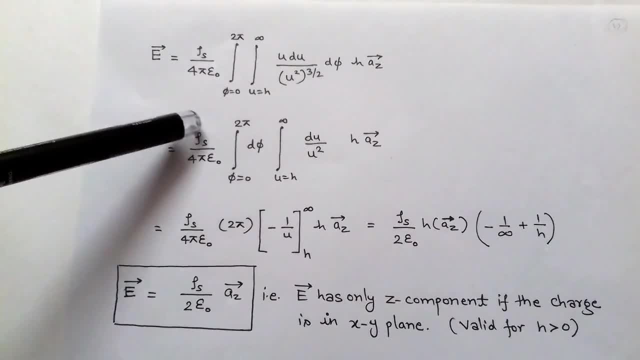 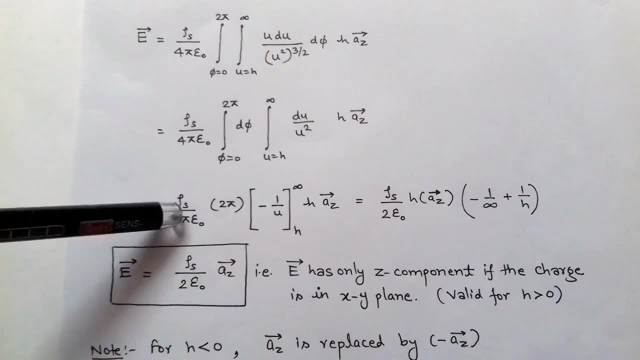 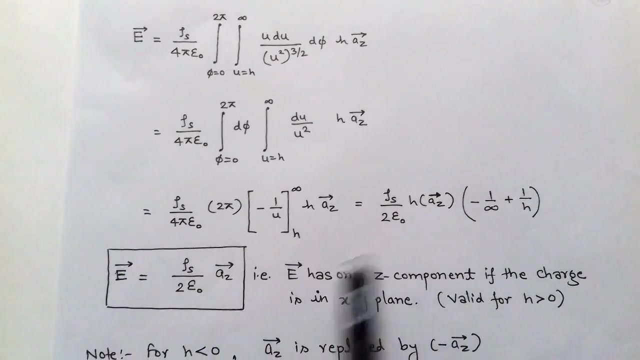 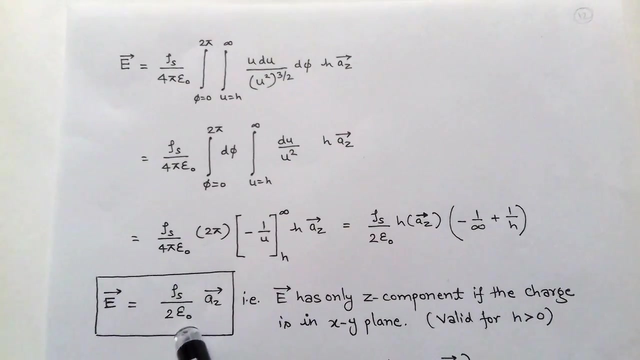 the phi part with respect to phi and u part with respect to u. now, after integration and putting the limits, we get electric field intensity that is Rho s upon 2 epsilon 0 unit vector z means this electric field intensity has only z component if the 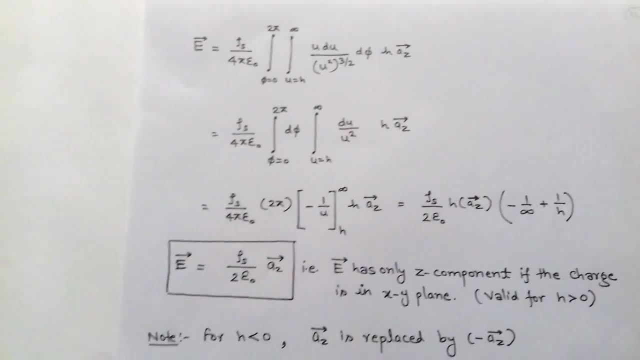 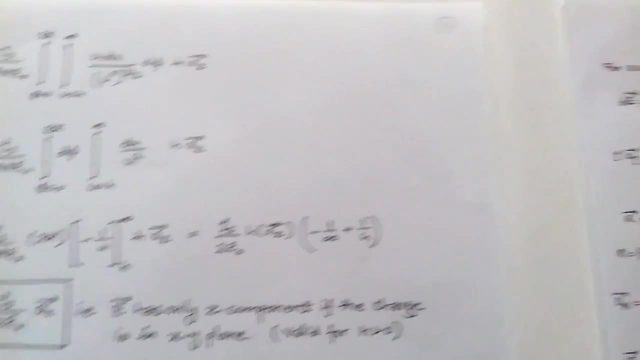 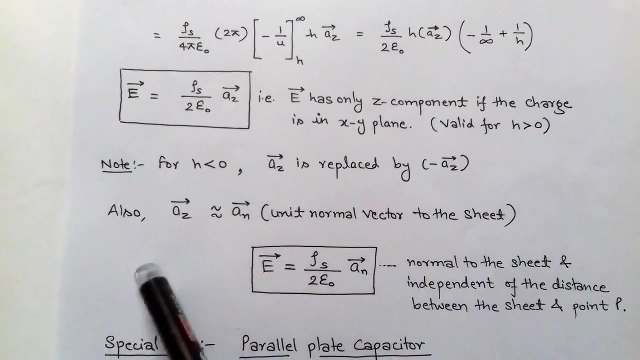 charge is in x y plane. this is valid for h. is greater than 0 means positive side for h, less than 0 for negative z. unit vector z is replaced by minus unit vector z, since this is a normal unit vector. so in place of unit vector z we can write normal. 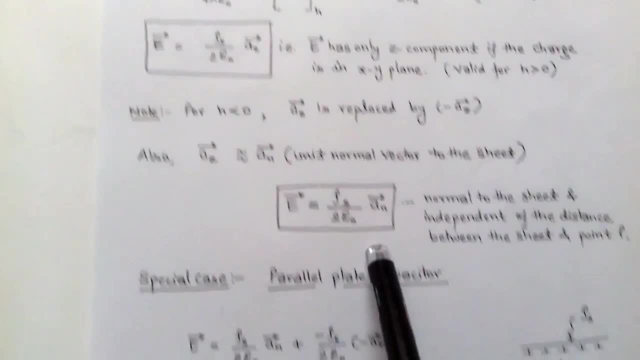 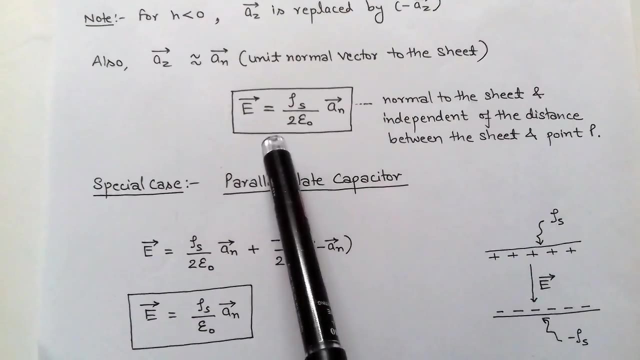 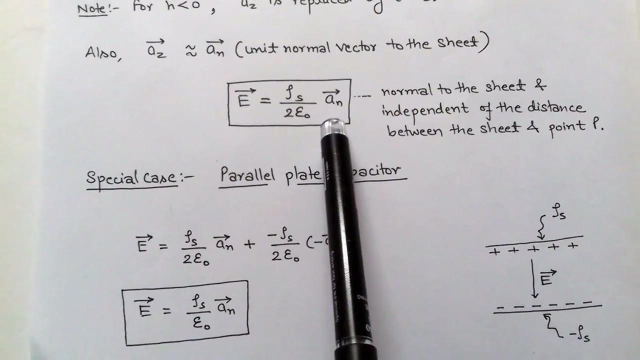 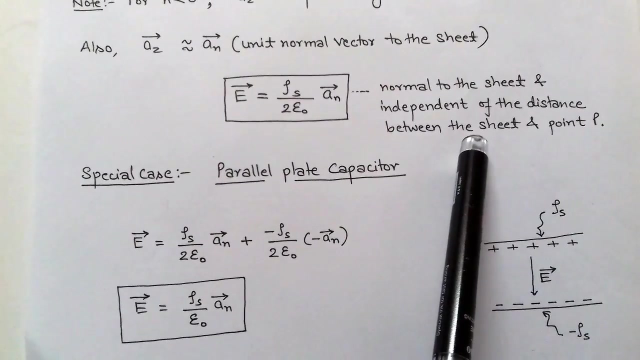 unit vector an. so this is a general formula for the infinite sheet that is electric field intensity e, due to an infinite sheet that is Rho s upon 2 epsilon 0, unit vector n, and it is independent of distance between the sheet and point p. now there is a special case. 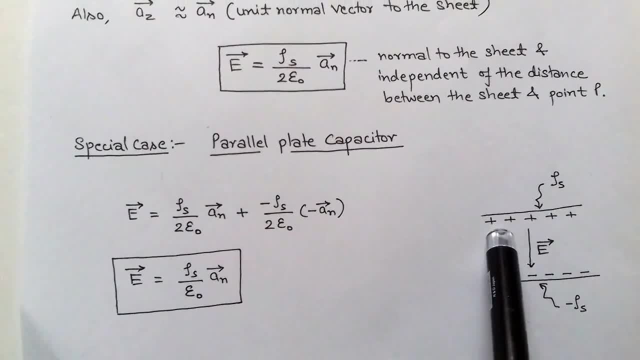 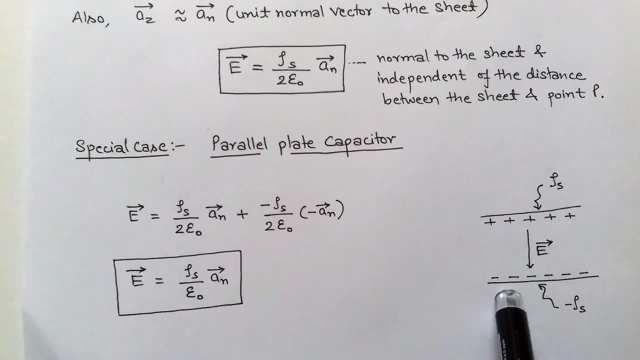 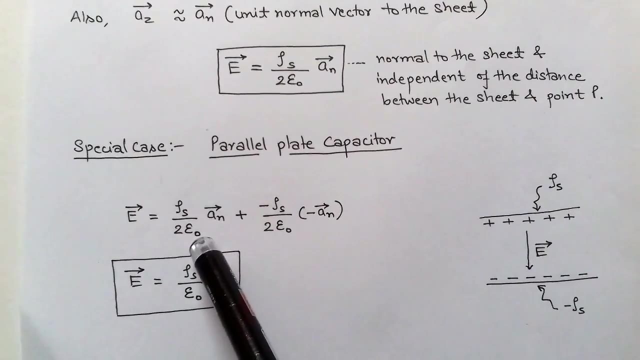 two parallel sheets. one carry a positive charge and another carries a negative charge, so the surface charge density for positive is Rho s and surface charge density for negative is minus Rho s. so due to this it makes a parallel plate capacitor and the electric field is generated from. 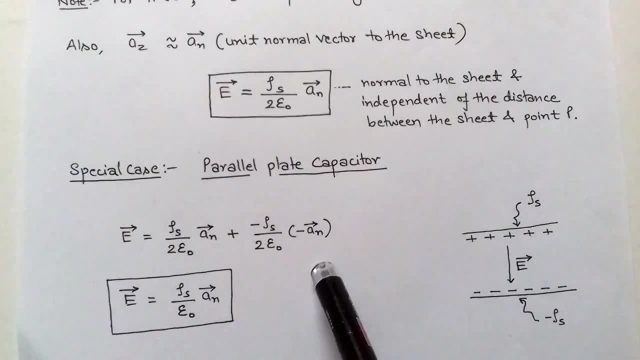 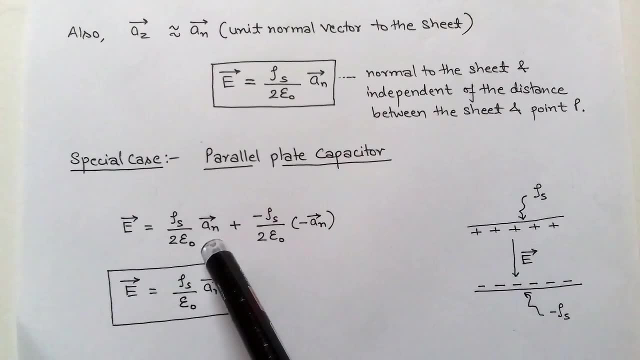 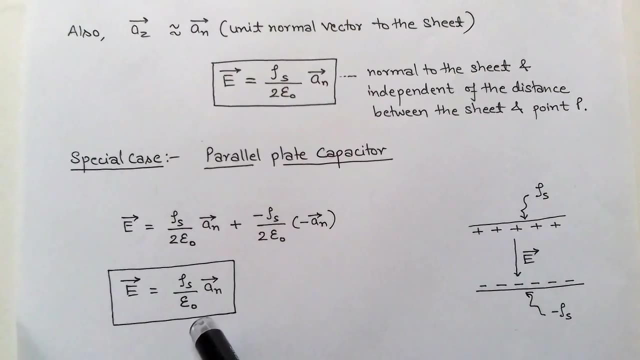 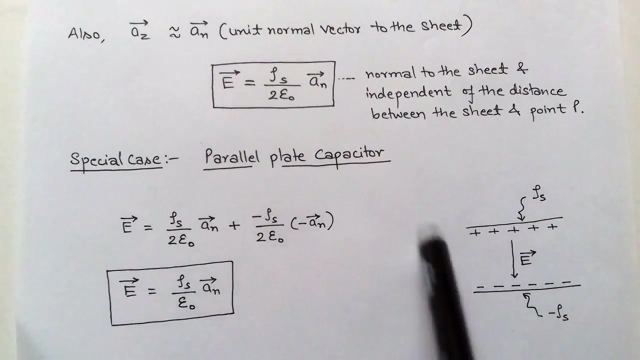 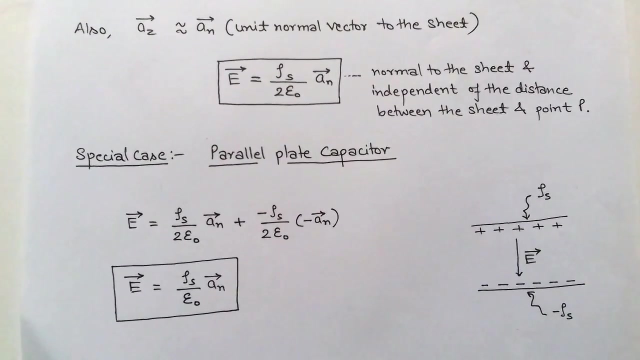 positive charge and terminate to negative charge. so accordingly the electric field intensity due to this parallel plate capacitor becomes Rho s upon epsilon 0, unit, vector n. here we consider a two sheet. so the formula is same, but the direction- normal direction- is opposite. so the electric field density due to 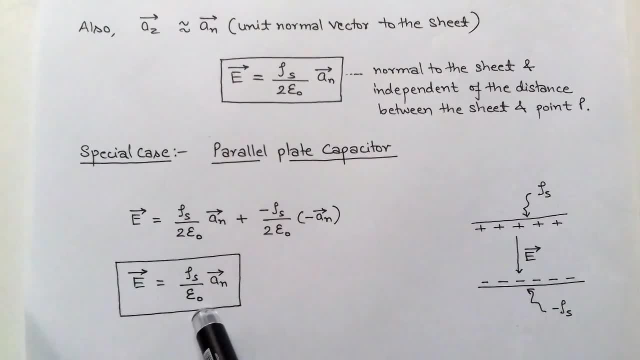 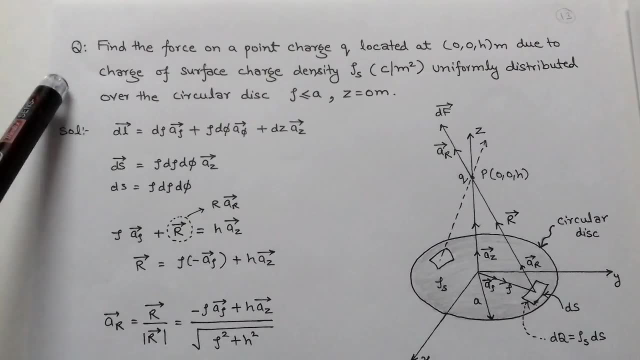 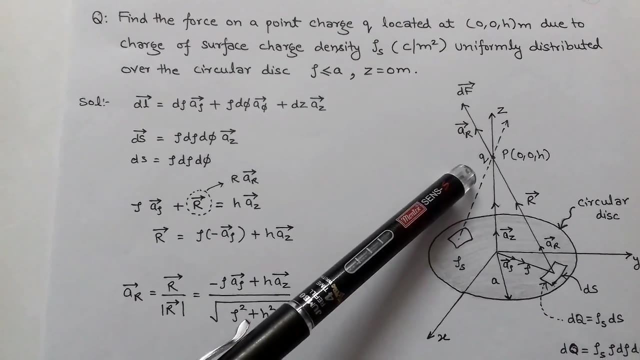 parallel plate capacitor is Rho s upon epsilon 0 unit vector n. now consider a numerical portion. the question is: find the force on point charge cube, small cube located at Rho h meter due to charge on surface charge density. Rho s unit is coulomb. 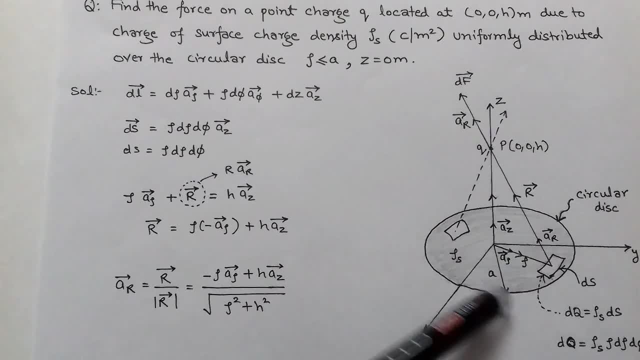 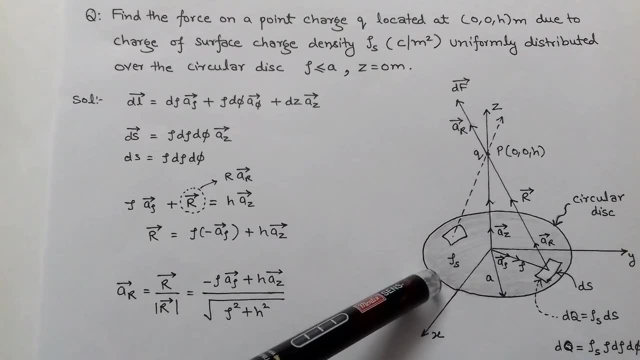 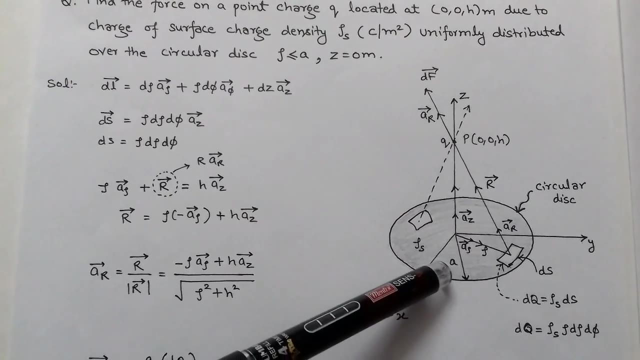 per meter square uniformly distributed over a circular disc Rho less than or equals to a and z equals to 0 meter. so, according to this question, there is a circular disc having radius a and that is situated on z equals to 0 meter, that is, on x y plane. 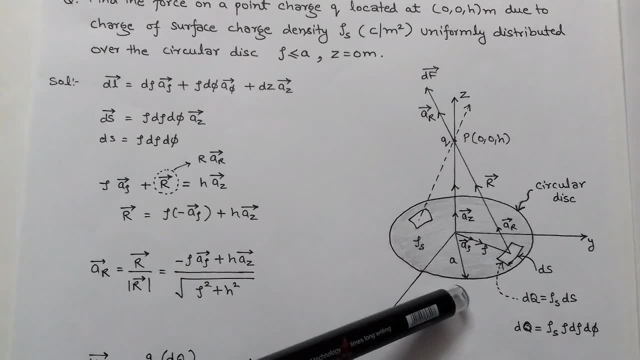 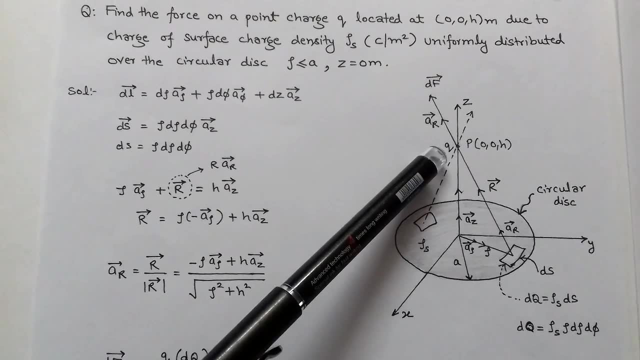 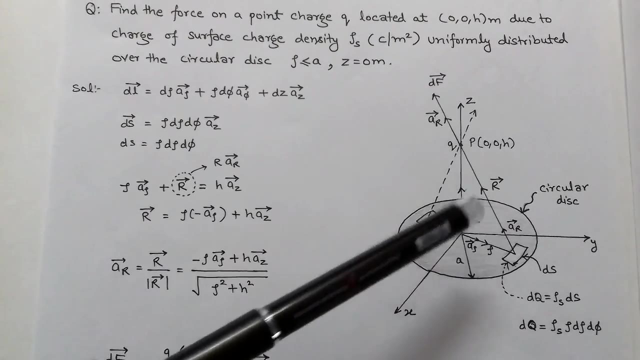 so there is a circular disc situated on x y plane and we have to find the force on point charge small cube that is located at 0, 0 s, that is, on z axis. ok, now the circular disc having a surface charge density Rho s. so this is a similar. 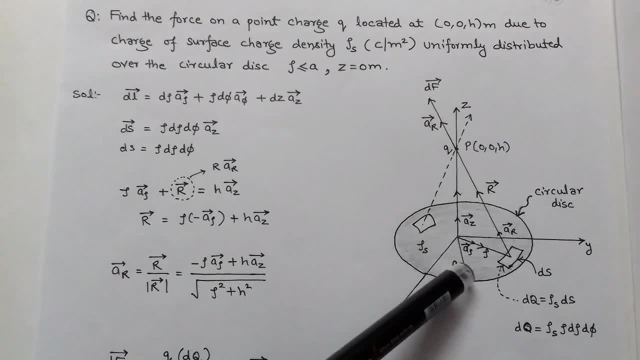 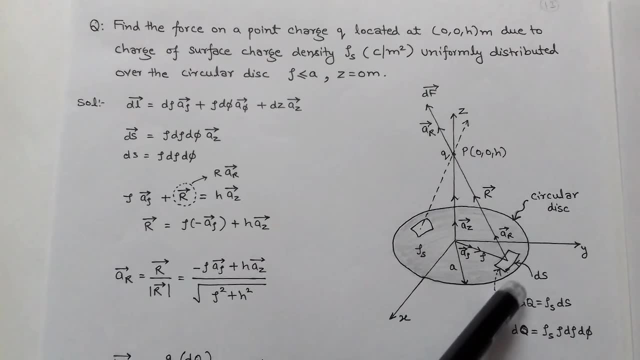 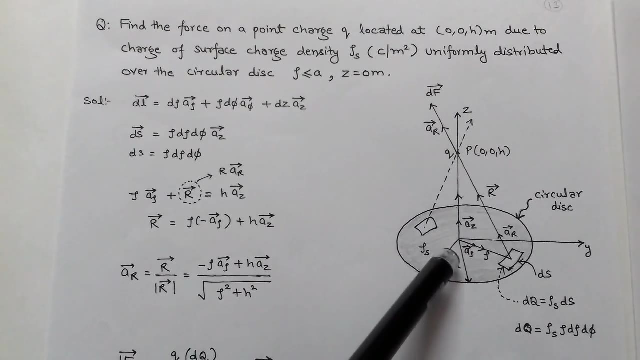 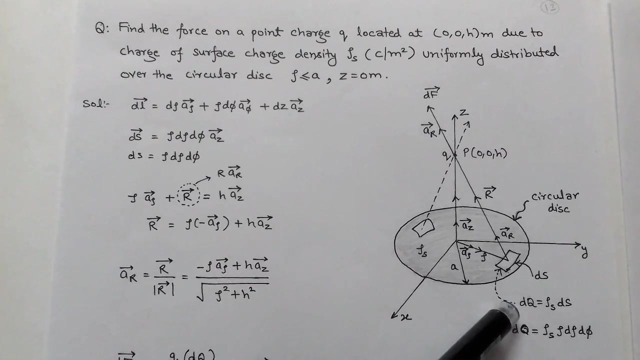 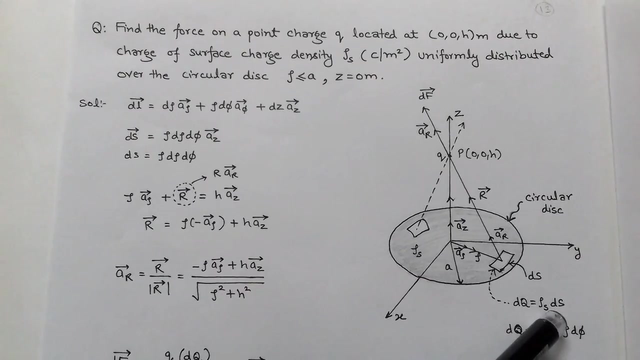 type question. now, first step is we have to consider a differential surface ds at some distance, Rho. this Rho makes some angle phi with respect to x axis. now this ds having a small charge, dq- that dq equals to Rho s- into ds. now, since ds 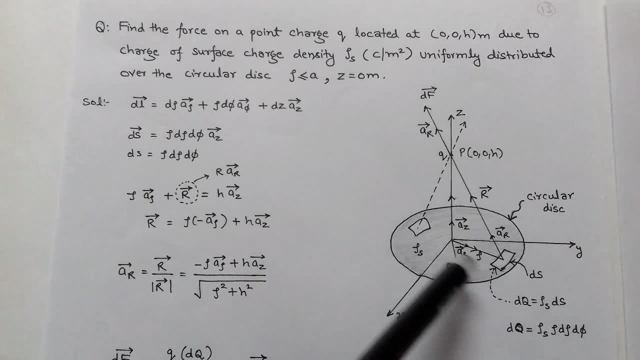 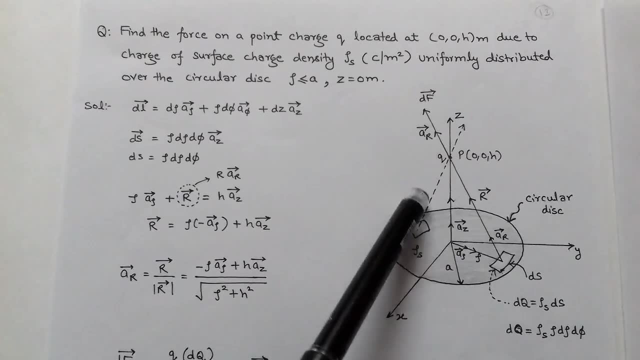 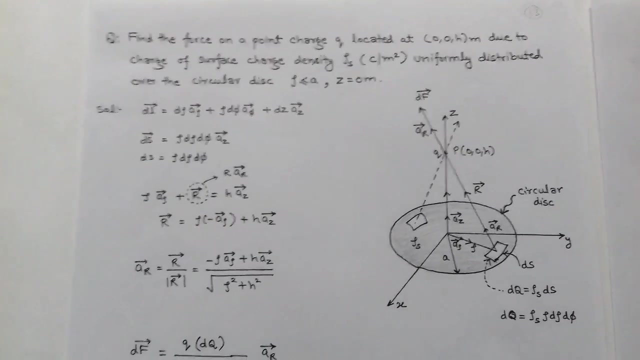 now this surface having a normal direction, that is, towards z axis. so the differential surface ds in the direction of z can be determined from the differential length that is Rho d Rho into d phi in the direction of z and the magnitude part is of ds. is ds equals to. 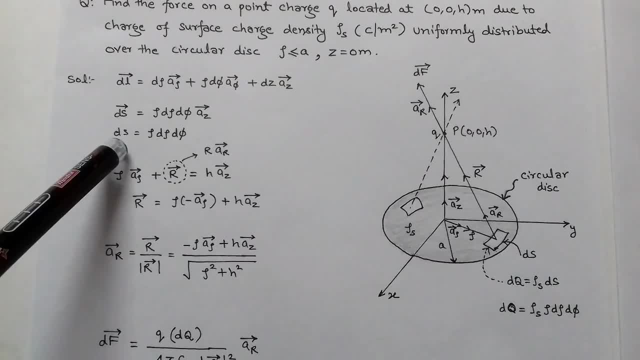 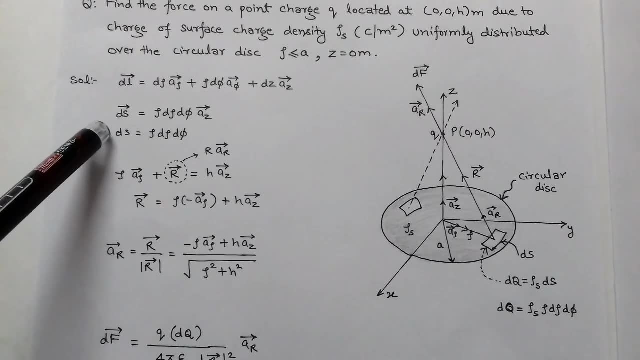 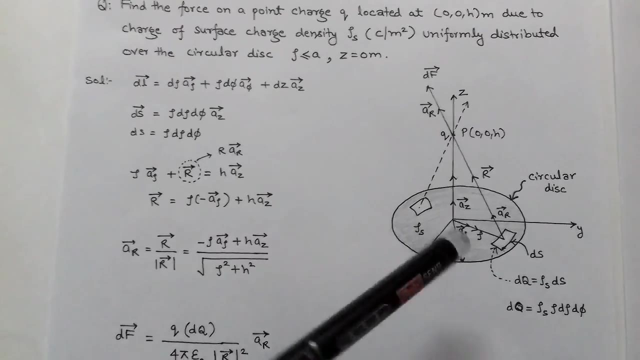 Rho d Rho into d phi. so in place of ds we can write Rho d Rho into d phi. now, this ds having a distance- Rho with respect to origin- and this Rho having a unit vector, A Rho. again, this ds is having a distance. 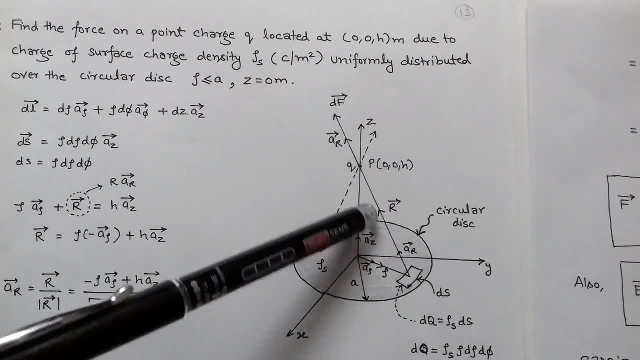 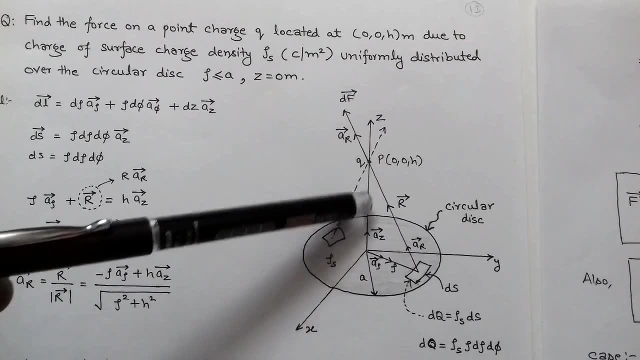 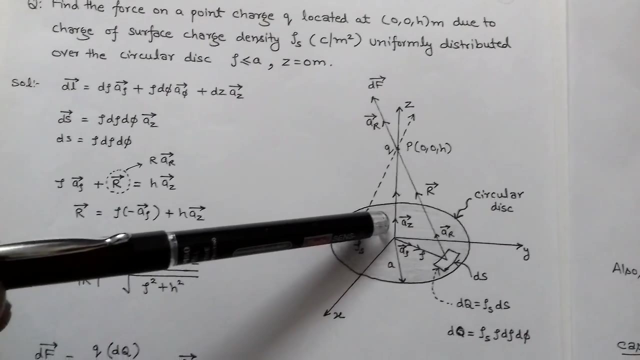 R with respect to point P. so here we consider a vector R having a unit vector A, R and this point having a height h and its direction is towards z axis. so here we consider a unit vector z, now using a vector sum. so Rho unit vector. 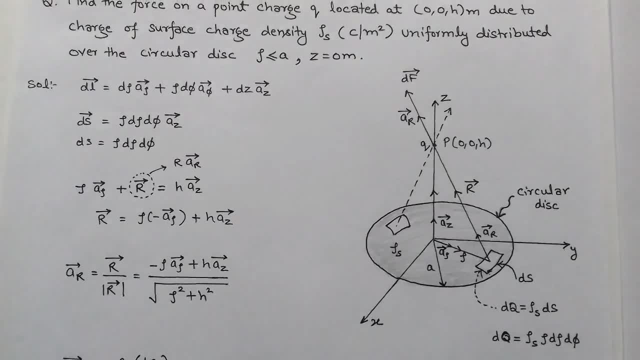 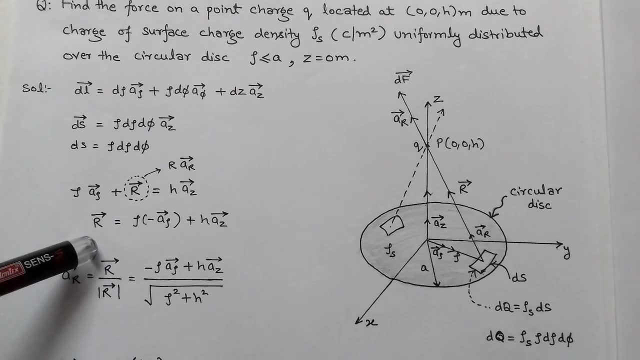 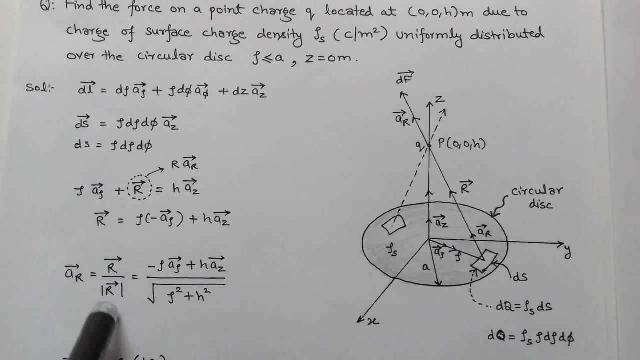 Rho plus vector R, capital R equals to h unit vector z. so the vector R equals to Rho minus A. Rho plus h unit vector z. so unit vector R, capital R, equals to vector upon its magnitude. so we use a force formula, coulomb force due to 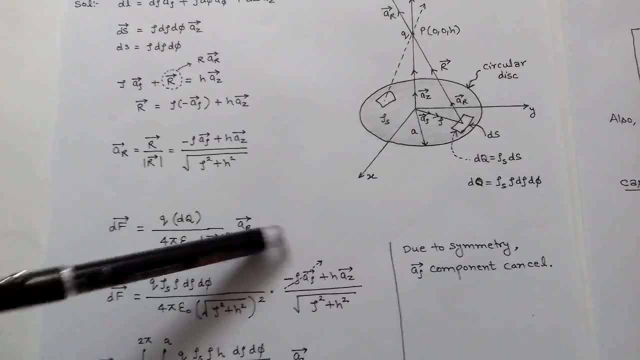 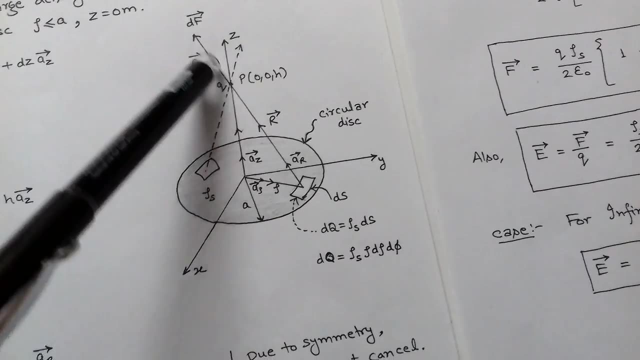 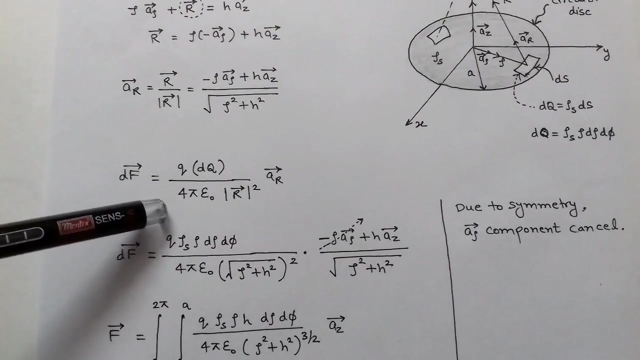 this ds there is a small charge, dq, and accordingly a coulomb force. both are positive so it is ripple force. so the small force df, equals to small q into dq. upon 4 pi, epsilon naught R square in the direction of R. so after putting these, 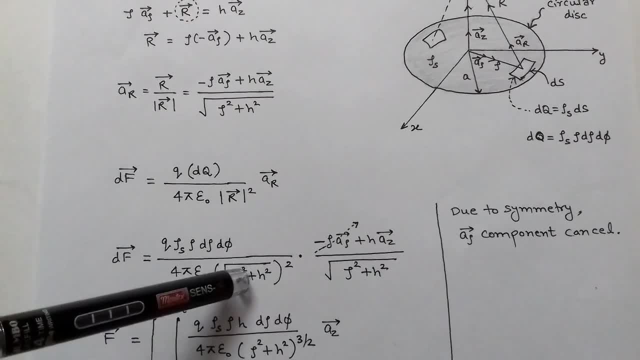 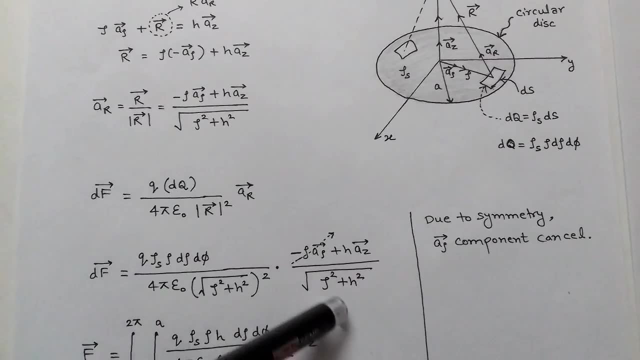 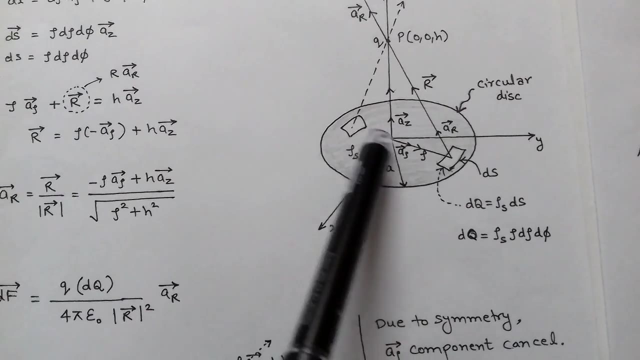 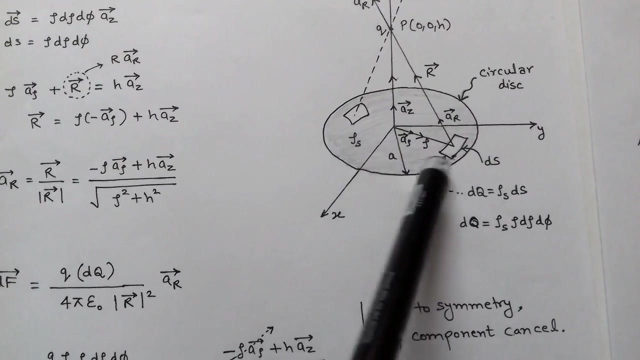 values, the value of dq, the value of R. we get this and in place of unit vector R, we can write vector upon its magnitude, since, due to symmetry, due to symmetry, the Rho component is cancel out for every element, there is an opposite element which whose effect is cancel with. 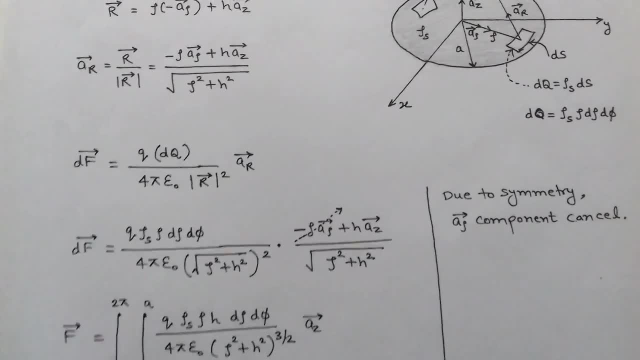 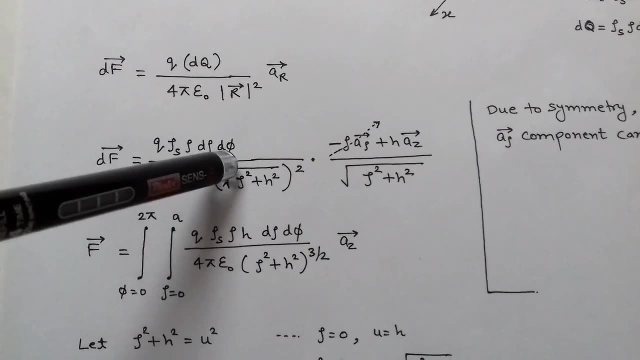 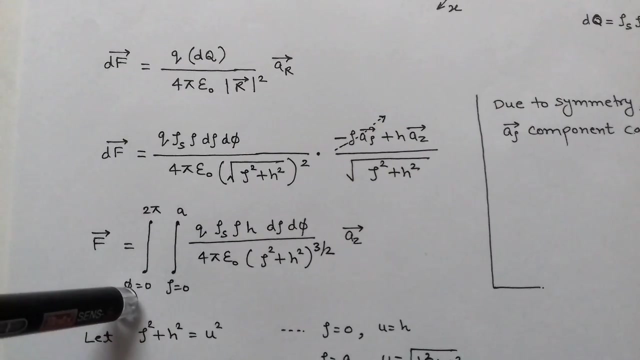 each other. so there is only z component here now. similarly, there are two differential term, dq, d Rho and d phi. so there is two integration. one integration with respect to Rho and second integration with respect to phi. the limit of Rho equals to 0 to. 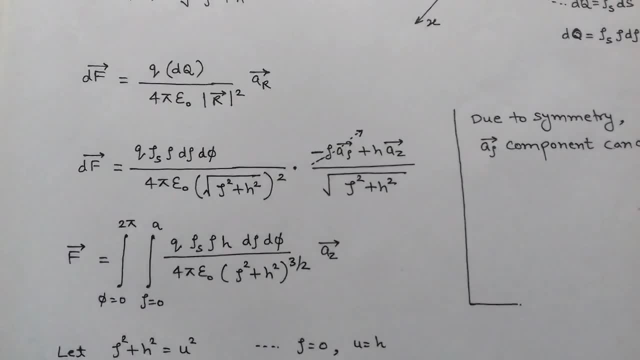 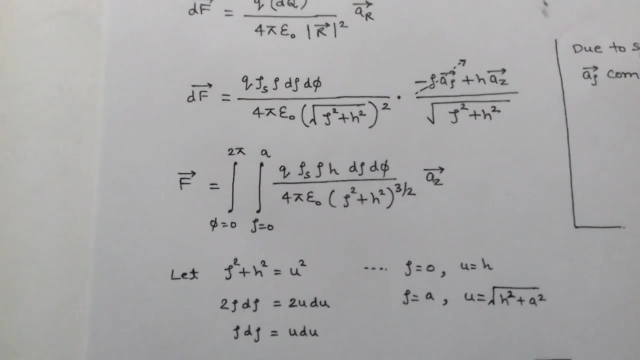 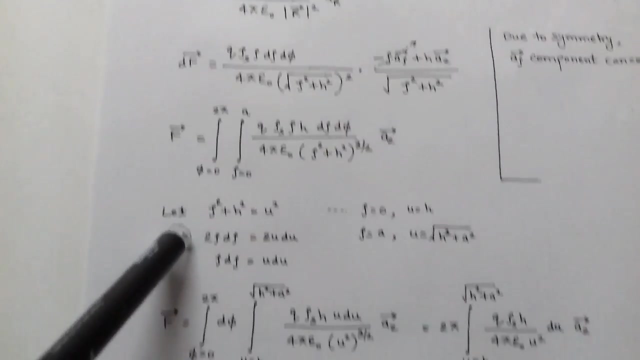 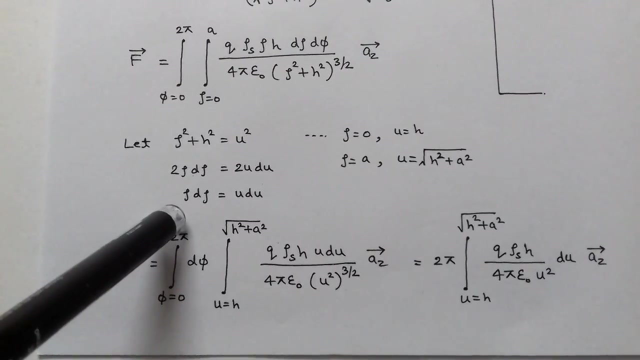 a, that is radius, and the limit of phi is from 0 to 2 pi. so here we assume that Rho square plus r equals to u square to calculate this integration. so 2 Rho d Rho equals to 2. u du two days cancel Rho d Rho equals to: